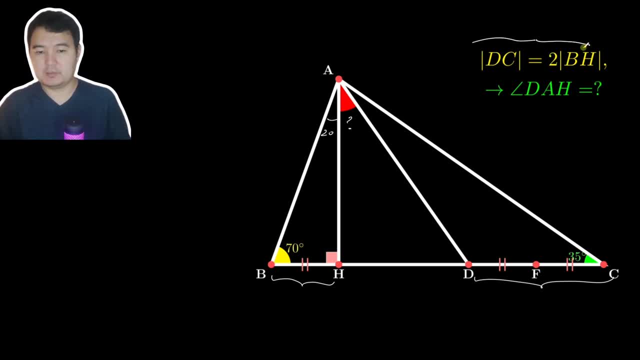 that's an information given, So we need to use that information somehow. Let's take this AB and put this AB here. So if you put the AB, take this AB and put it here, So these two are equal and what that gives you. So how do you get this idea? The idea comes from that. 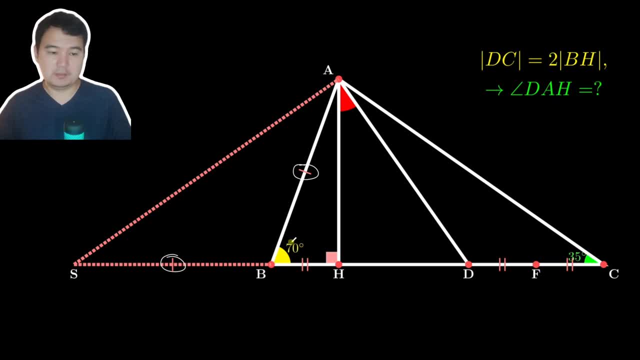 we have 35 degrees here and 70 here, So this will be isosceles triangle with 35 degrees over here and another 35 degrees over here, because 35 plus 35 will be one exterior angle, 70 here. And then another interesting observation is that we have this triangle the large. 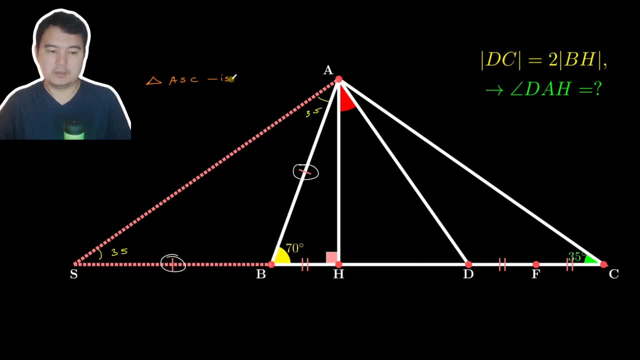 triangle ASC to be isosceles, because 35 degrees here and 35 here. so we could say this one isosceles is equal to this one, but we are not going to use it anyways. however, we know that the altitude of isosceles triangle, this altitude of the isosceles triangle, is also median because it's isosceles. 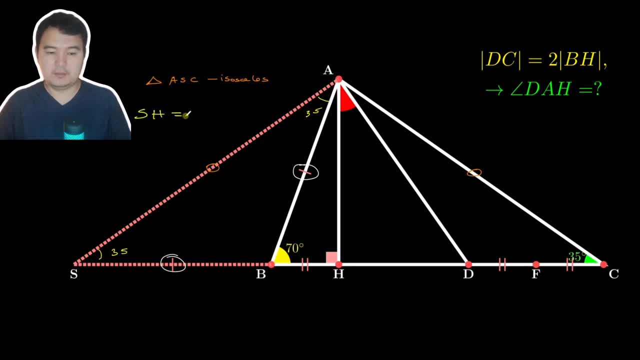 so that gives you sh is equal to hc. so this is a very useful information. okay, let's say this is 20. we have this information here because of 70, 90 and this 20. now let me put x here, the length of bh and then the length of this one, and this one will be x as. 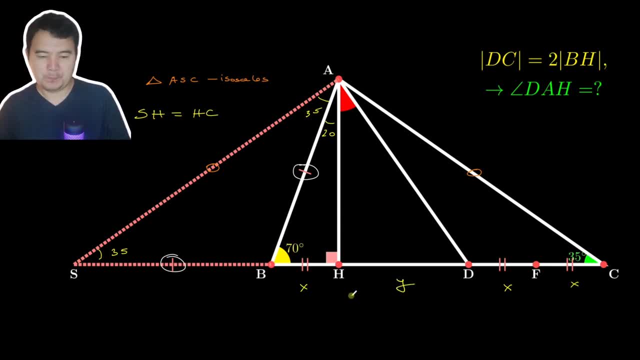 well, and let's say this is y. the total over here hc is 2x plus y, so we need 2x plus y for sh as well. so that's x plus y. so total we have 2x plus y. since this is x plus y, 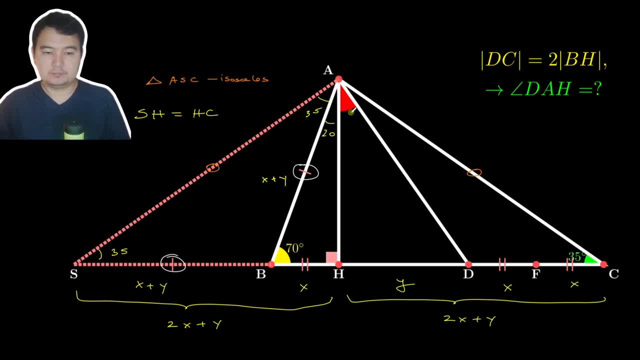 this one is also x plus y and this part of bd. so if you pay attention to bd this it's also x plus y, so the triangle abd. so this triangle is an isosceles one with the sides x plus y here and x plus y here. 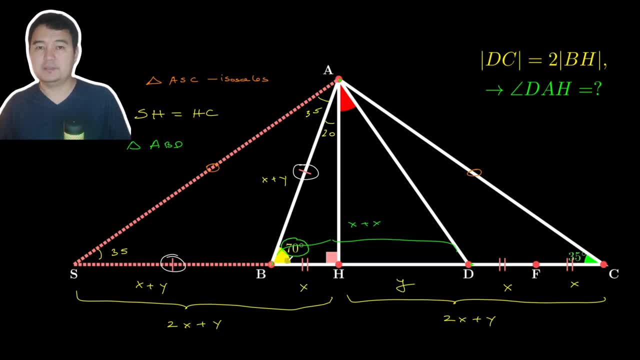 and with the angle 75 on the top. so what will be the other two angles? so that will be 70 plus 2x, let's say 2. let's say 2, alpha is 180 and alpha has to be 55. so in order to get the 55 degree angle here, i need 35 and 55 here. so the angle that i'm looking. 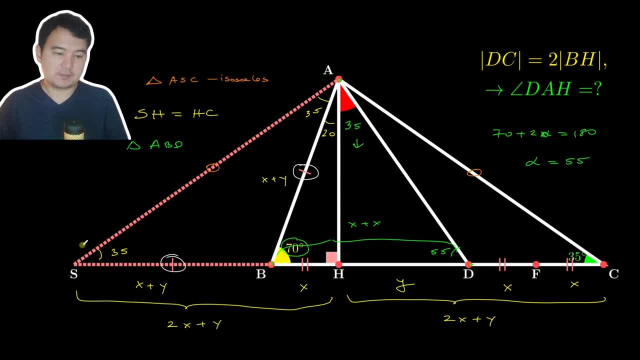 for is 35, so adding this extra construction over here makes the problem much more easy. 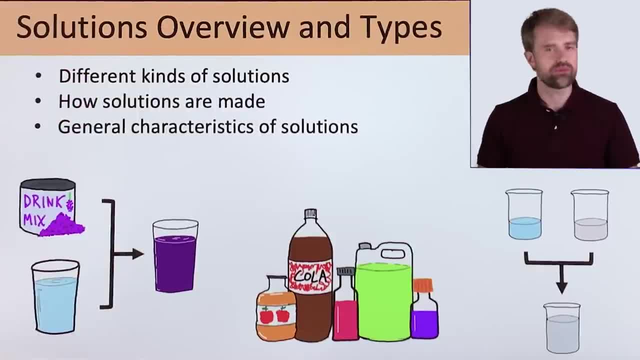 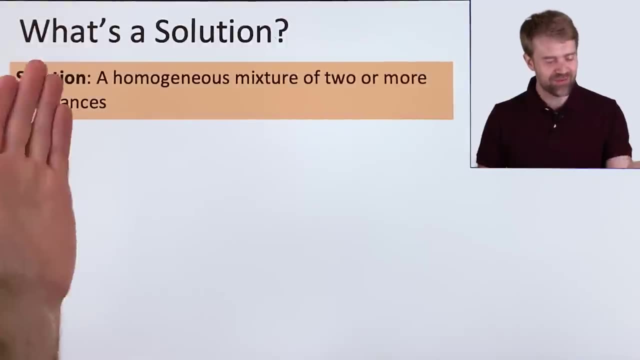 In this video we're going to take a look at solutions which are a type of mixture used a lot in chemistry. We'll look at some different kinds of solutions, we'll see how they're made and we'll look at some general characteristics that all solutions have. So to start off with what's a